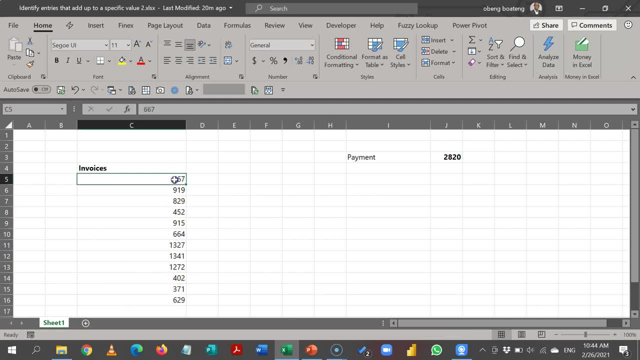 So question is: which of these numbers can sum up, or which combination of these numbers can sum up, to give us this payment. Now, to do this, we are going to add a few things. So the first thing we are going to do is to create a helper column against these invoices. So let's. 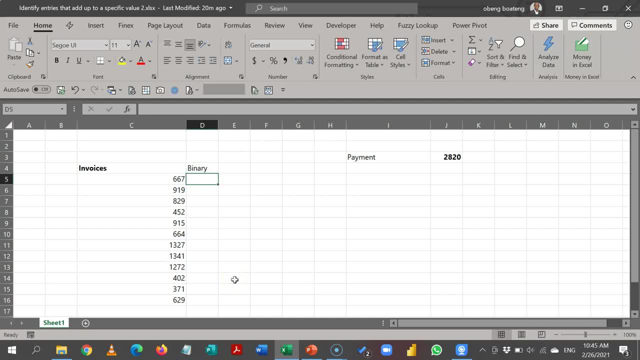 call this binary, And we are just going to highlight these and then fill these cells with one. Okay, so these are the values that are going to help us calculate To get a sum that matches this. Now, to do this, we are going to multiply each row and then sum up. 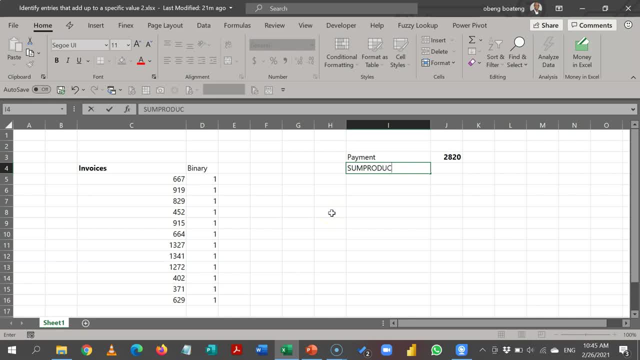 There's a function to do that, And that is some product. So some product allows you to multiply C by D And when you are done you sum up whatever you have. It's a very simple formula, yet very powerful. So equal to some product, And I have two arrays. It's important. 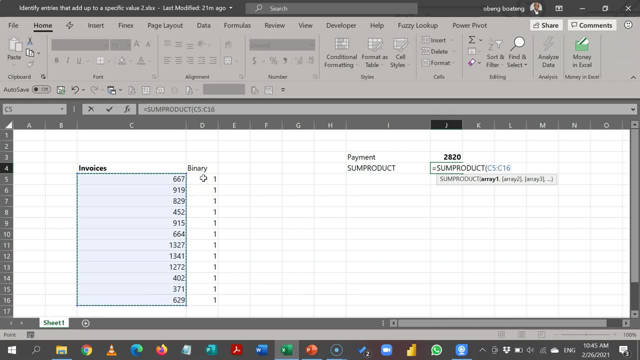 that the two heights are the same. So my first array is C15 to C16. And my second array is this: D15 to D16. So when I do this, currently all the invoices sum up to 9788.. Now the third thing. 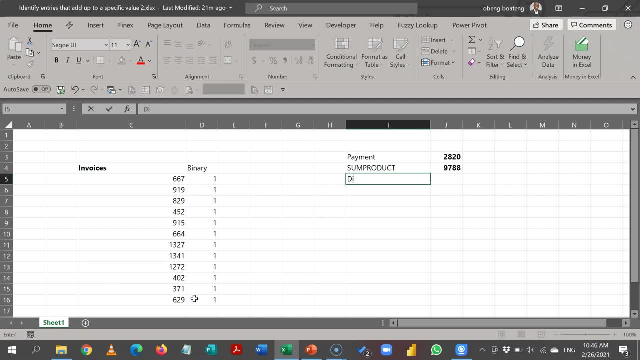 you're going to do is just to find a difference, And this difference is going to be your objective In the end. we want this to be zero, So I'll just take this: Minus that, And we have this 6968.. Now to make it easier for you to visualize what is going to go. 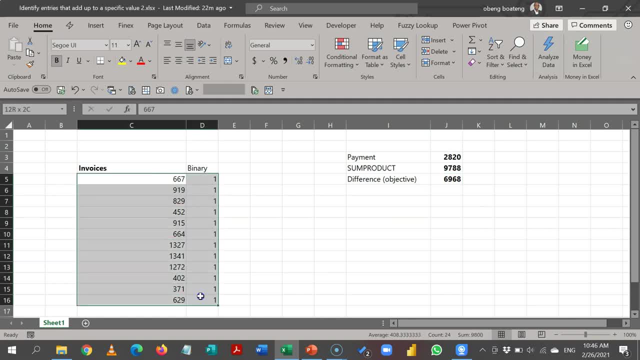 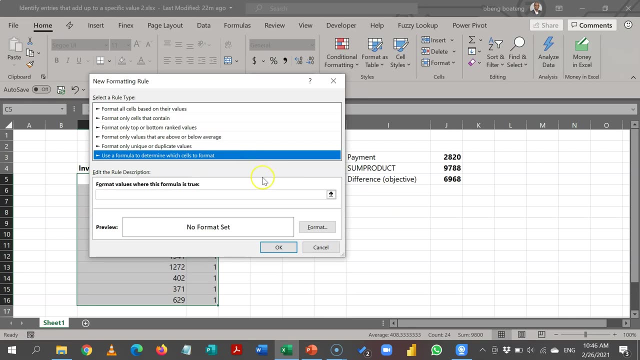 on. I'm going to apply a conditional format to this range. Okay, It will highlight each rule. if, in the end, what ends up in this range is going to be one, So I'll highlight. go to new rule. use a formula to determine which. 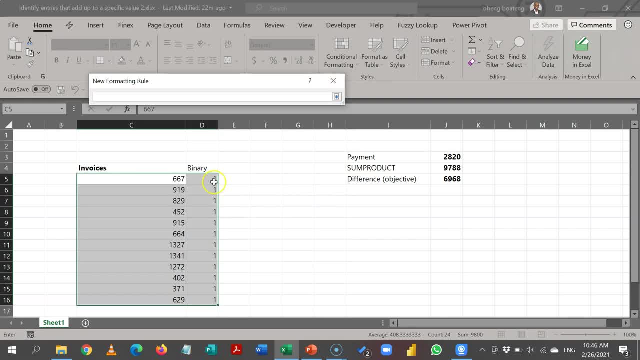 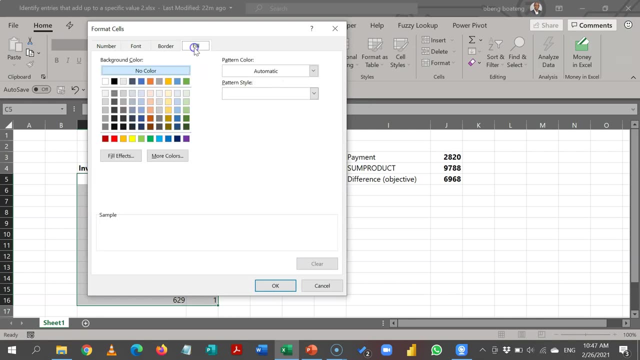 which area to apply. my condition Now format. And then I'll say: if D5, F4, F4, so that the rule is free and only the column is locked- is equal to one, Then what happens is: I want to apply a light green format. 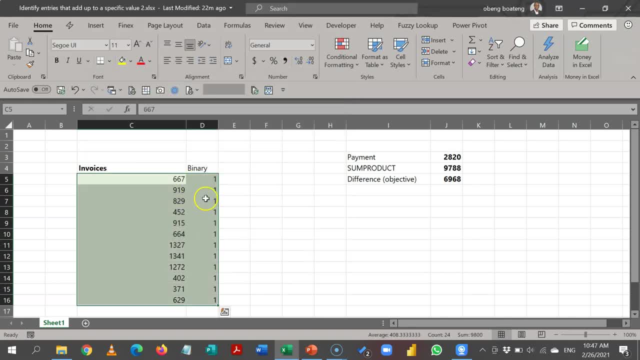 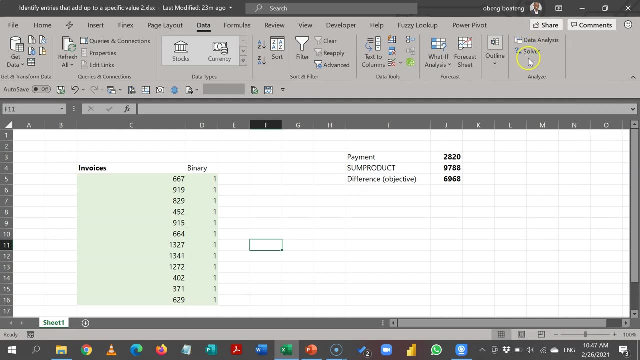 Okay, And then I click OK. I expect the whole thing to be highlighted. In the end, the answers will only be highlighted, Okay. So now that we have this, what we are going to do is to activate our solver. Solver is under data And in your stream right is part of the add-ins, So 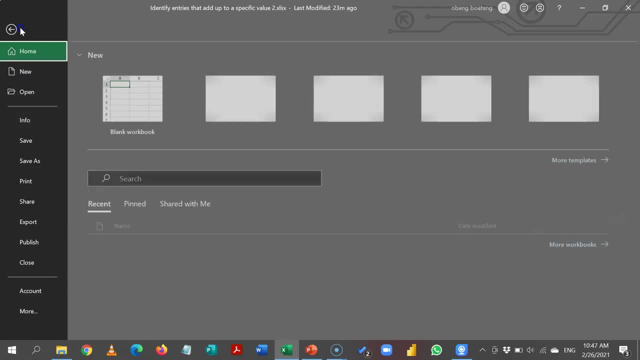 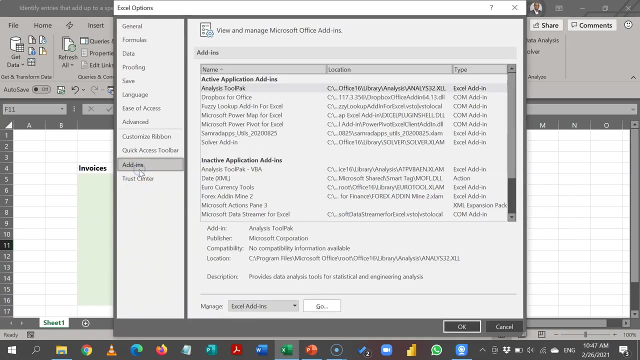 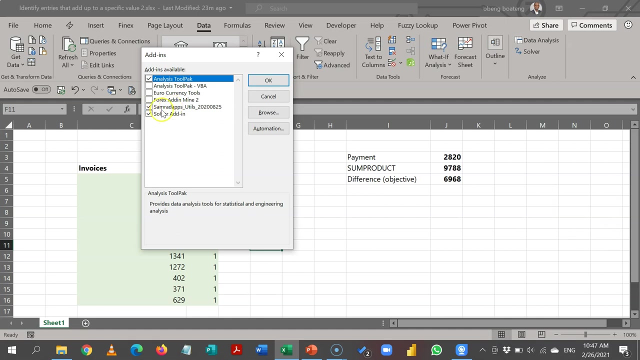 solver should be here. If you don't have it, you can go to file options and then add-ins And then you choose Excel add-ins go. Then you check the box for solver. Another shortcut is Alt T- I, which just brings up this add-ins dialog box. So you check the box and it activates. 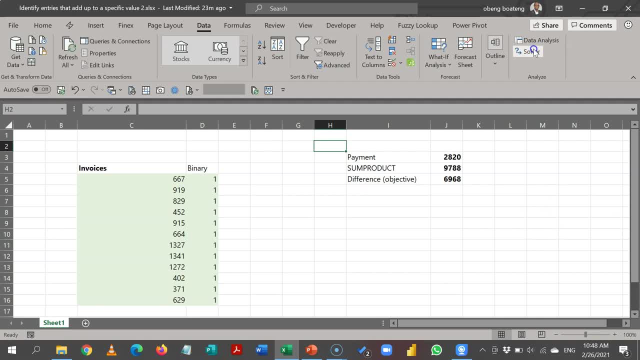 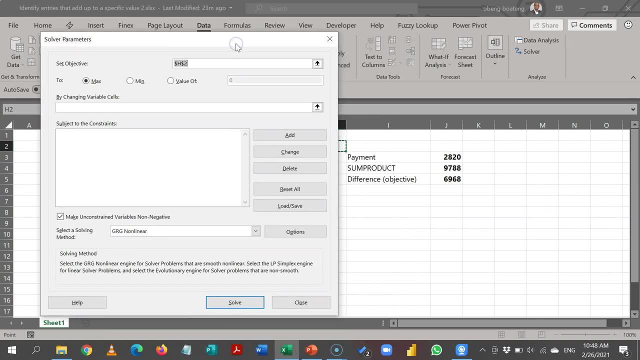 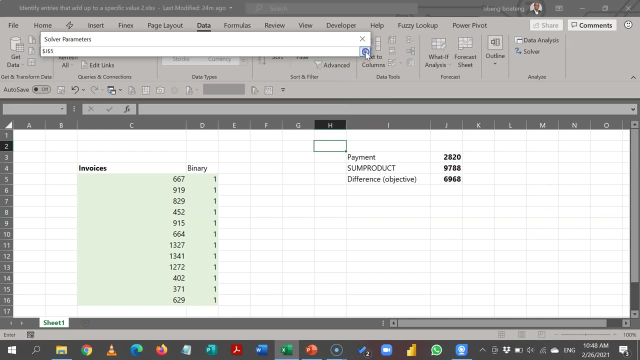 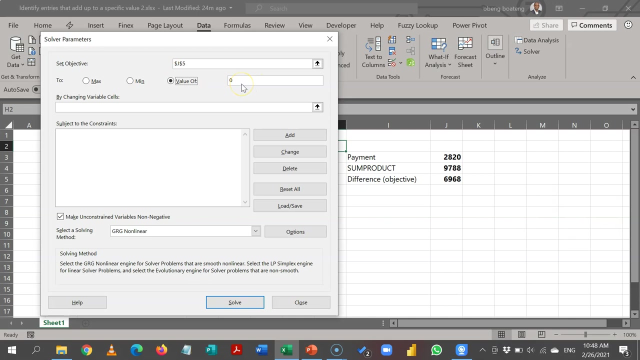 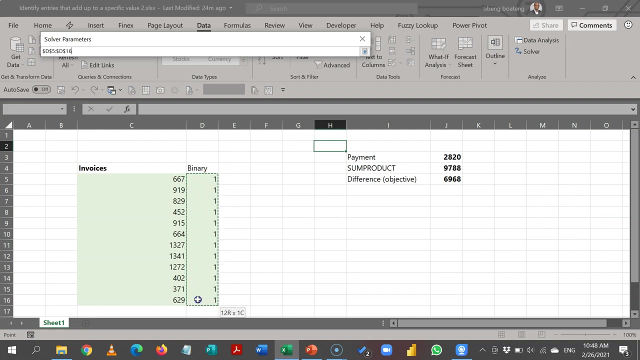 So it's a pretty simple process. Once we activate, Solver requires a set objective. So our set objective is to make cell J4, which is our difference, J5, I must say set it to a value of zero. okay, by changing these binary numbers in this range which is d15 to d16. 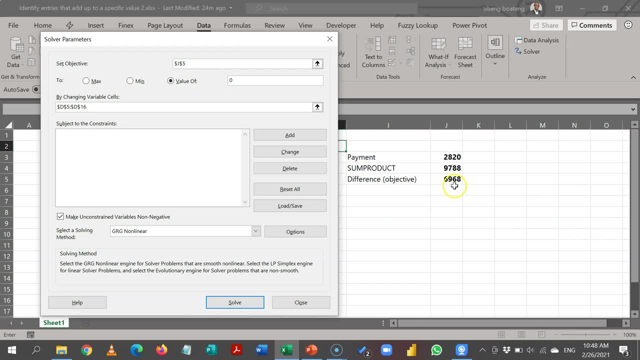 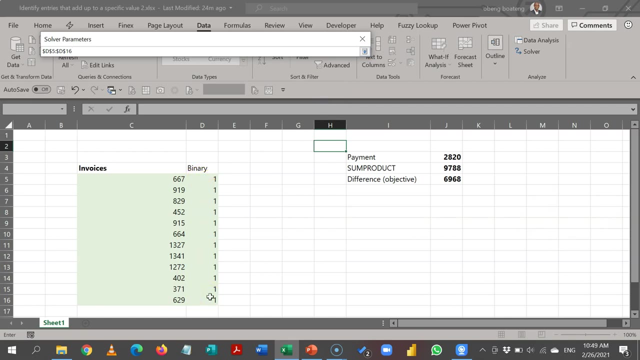 okay, so set this to a value of zero by changing d15 to d16. now you can solve with the constraints. we don't want anything that is greater than one and less than zero, so we are just restricted to ones and zeros. now, to do that, you can add a constraint and then we'll say this particular: 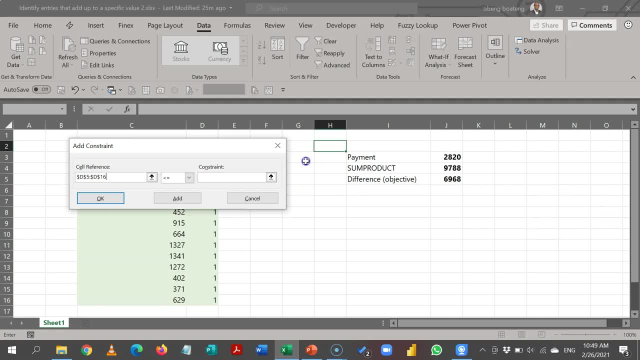 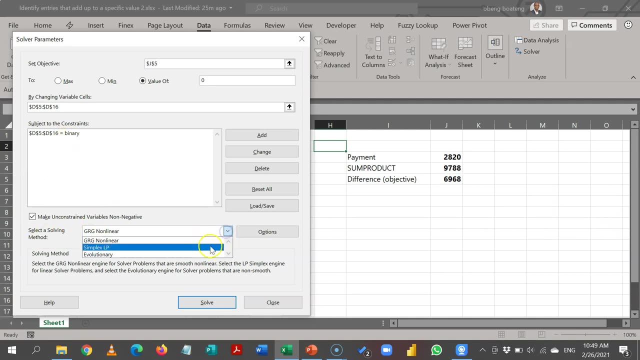 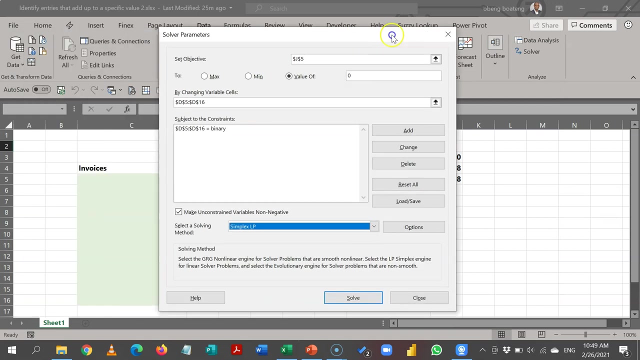 range for our binary numbers should be just bin, which is just binary. so once you add this, then you are fine. so this is our constraint and then we'll choose a solving method. we'll choose a simplest LP and then, once you are done, let me move this here so that you see what happens. so I'm ready to solve, then I click.